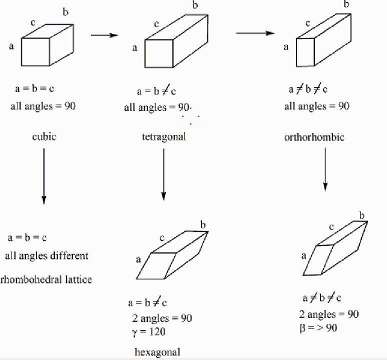 do in order to create the pattern for your wallpaper? What you would be doing is to draw enough of the picture that you could then use a cut and paste option to paste an image next to its neighbour so that you can build up the whole structure of the wallpaper. This 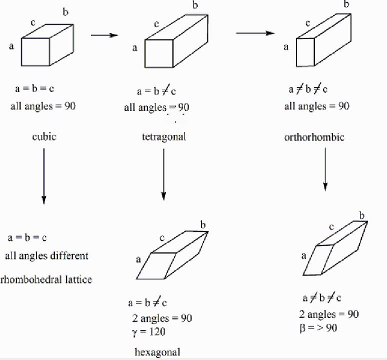 would be called the unit cell. So when you look at a crystal structure in three dimensions, the smallest size of the repeating unit is termed the unit cell. It must repeat exactly. The various shapes of the unit cell have been broken down into some standard shapes and we're going to look at those right now. 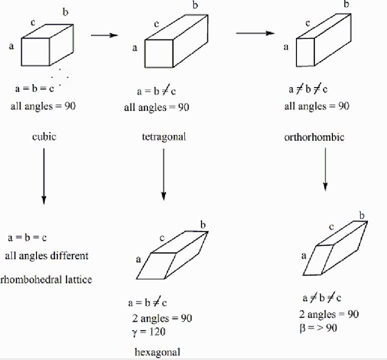 The very simplest is the cube, and that's where we have three sides, A equal to B equal to C, and the angles between them are all 90 degrees And the angle alpha is the angle between B and C, The angle beta is between sides A and C and the angle gamma is between 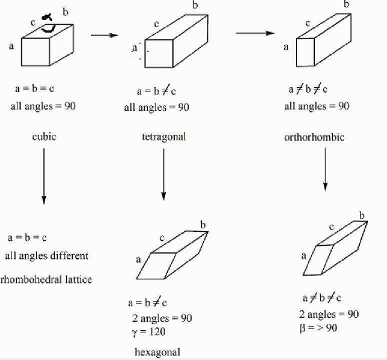 sides A and B. Now if we were to lengthen side C, then we will get this tetragonal shape. Tetragonal is where we've got two sides equal to one side. So we've got two sides equal in length and one side different, but all angles are still. 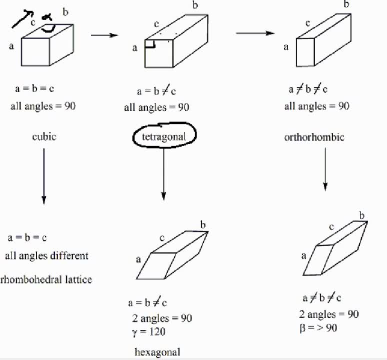 90 degrees, And so we can consider that the angles are still 90 degrees, like that, If we were to change the side of B. so, for instance, let's go for a contraction in this case could equally have been a lengthening, but just let's make all three sides different. 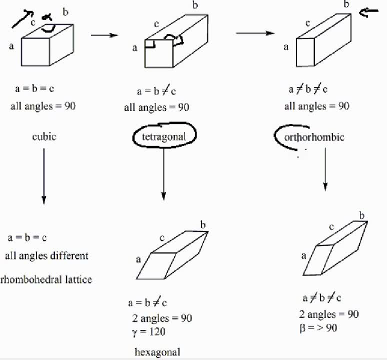 All angles still 90 degrees, then we end up with an orthorhombic pattern. Now we're going to do something rather tricky. We're going to push down on this particular edge and push it away from us, so that the angle here, which is the angle between A and